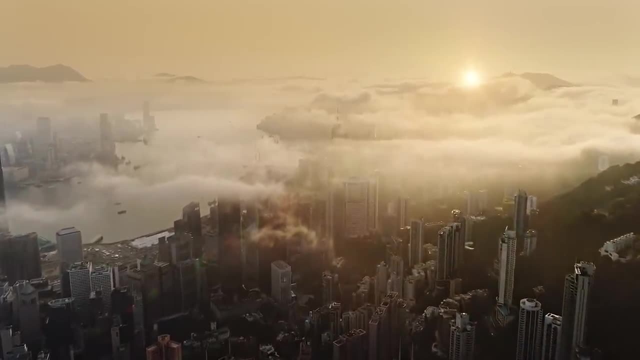 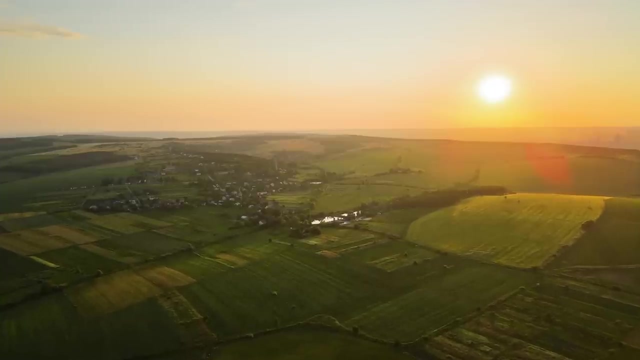 living in a city where there's lots of cars and things like power plants and refineries means you might have some ground ozone problems on hot, sunny days. But before you breathe a sigh of relief for living in a rural area, ground ozone gets blown around and transported by the 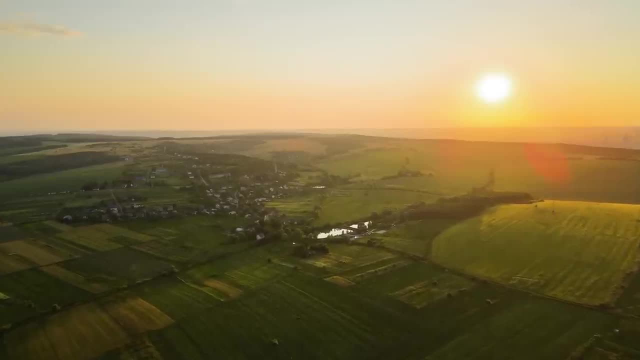 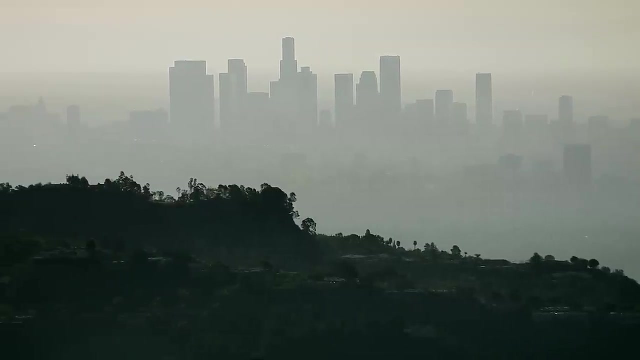 wind ending up in places that don't have things like lots of cars and refineries. Smog, a portmanteau word for a mix of the words smoke and fog, is a major form of air pollution. Any guesses on the main? 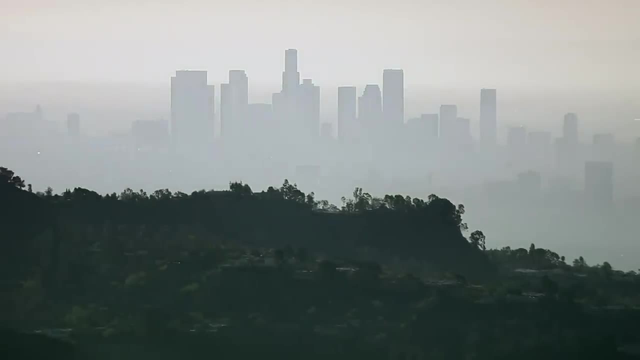 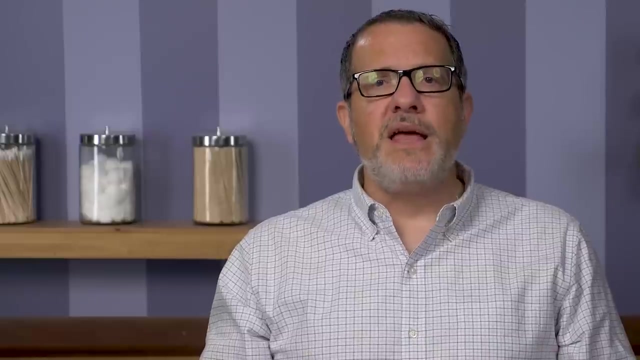 ingredient of smog: Ding, ding, ding. that's right, ground level ozone. So what's the big deal about it? Well, breathing the stuff in is pretty hard on the lungs and the lining of our airways. It inflames those airways much like a sunburn inflames our skin. It can cause the muscles in our airways to. contract which leads to trapped air in the tiny air sacs in our lungs and that makes breathing super hard. Taking deep breaths or breathing hard like during exercise can become difficult, even painful. It's bad for anyone that breathes it in, but especially bad for those of us whose lungs are already. compromised. for those suffering from various lung diseases, Breathing in ozone can make breathing a bigger issue than it already was. It can cause asthma attacks to happen more often and can aggravate conditions like emphysema and chronic bronchitis. It can also be especially hard on 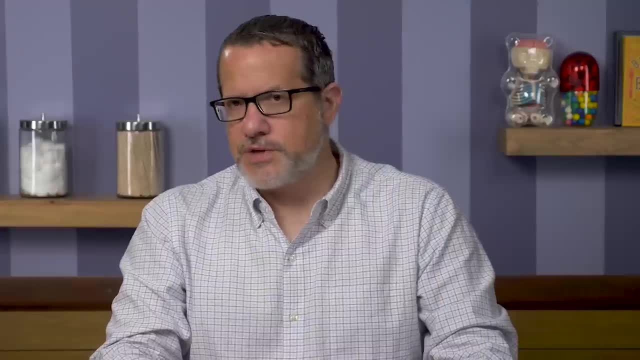 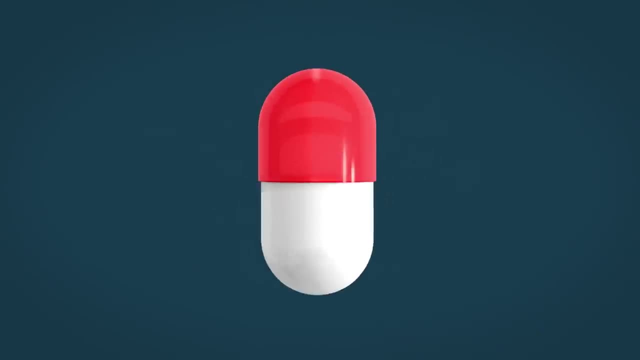 kids and elderly individuals. It's also possible that ozone does more than just aggravate asthma. in some cases, it could also be a factor in the development of the disease and other lung diseases. Other impacts of exposure to ground ozone include respiratory hospital admissions. 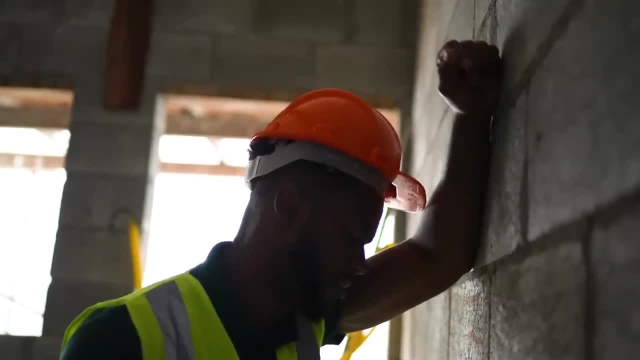 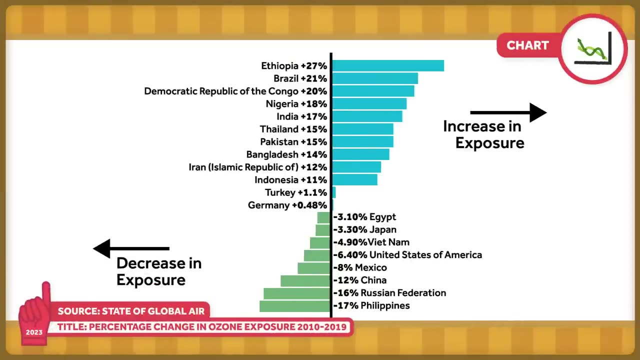 increased school absences, detrimental effects on outdoor workers and even premature death, And this is already an issue in many places around the world. Among 20 of our most populated countries, 12 have already seen increases in ozone exposure since 2010.. 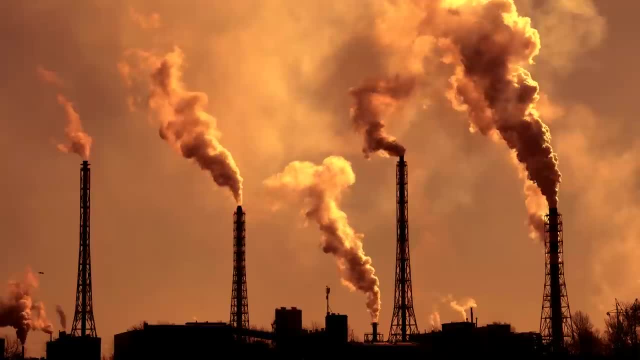 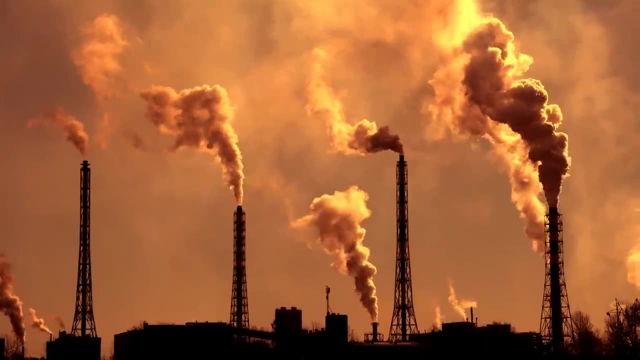 But wait, what does all this have to do with climate change? Emissions from processes such as the burning of fossil fuels are responsible for forming ground ozone, and those same processes are major contributors to climate change. Then, as climate change makes, 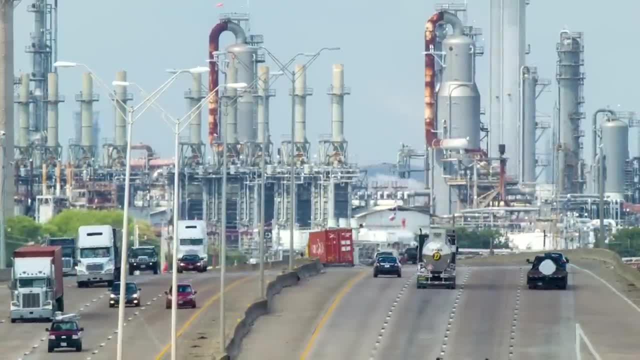 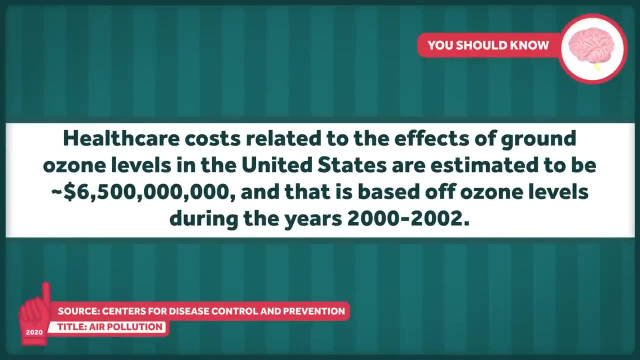 the air warmer and warmer, the chemical reactions that create ground ozone begin to increase. It's a terrible relationship and it's bad news for our health. Healthcare costs related to the effects of ground ozone levels in the United States are estimated to be somewhere around $6.5 billion, and that's based off ozone levels. 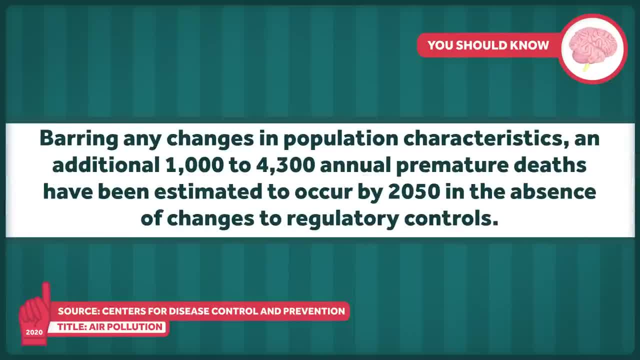 during the years 2000 to 2002.. Barring any changes in population characteristics, an additional 1,000 to 4,300 annual premature deaths have been estimated to occur by 2050 in the absence of changes to regulatory controls. Unfortunately, that isn't the only pollution-related. 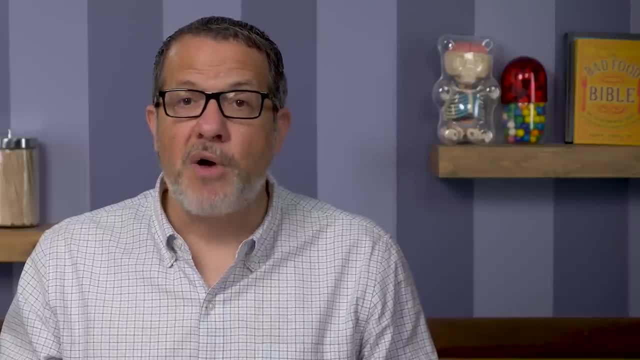 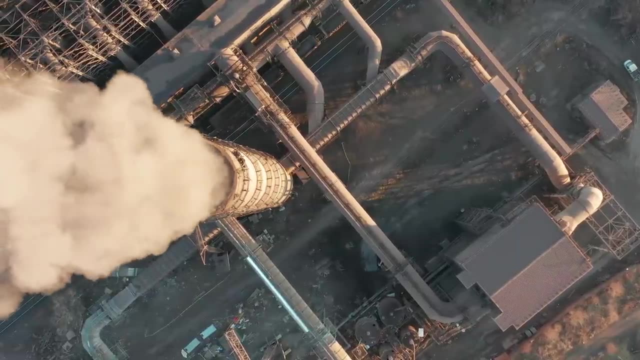 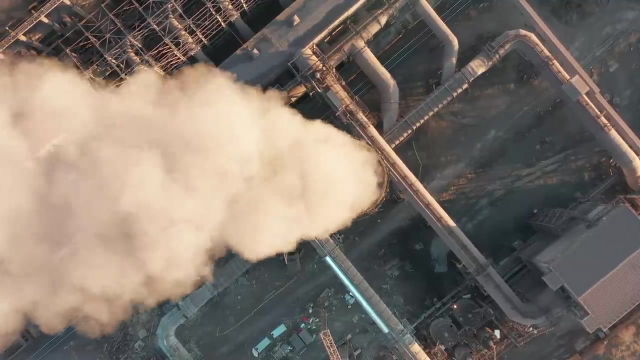 health concern to worry about here. Climate change-induced increases in particle pollution are also a considerable health threat. Particulate pollution or particulate matter consists of very small liquid or solid particles suspended in the air. These particles are very large and they can float in the air. Some of these are large enough to see like smoke. 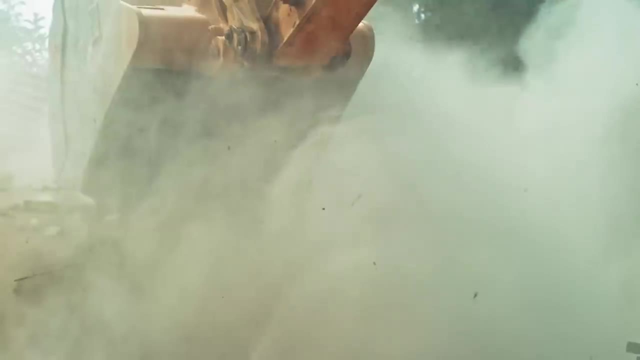 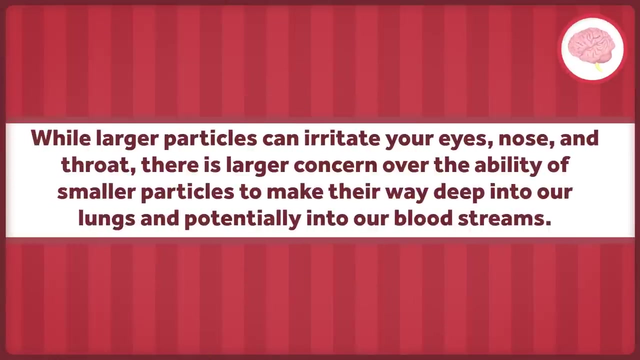 while others are so small that we can't see them floating around. These may include things like dust, dirt, soot and drops of liquid, Seen or unseen. this type of pollution has serious health effects. While larger particles can irritate your eyes, nose and throat. there's larger concern. 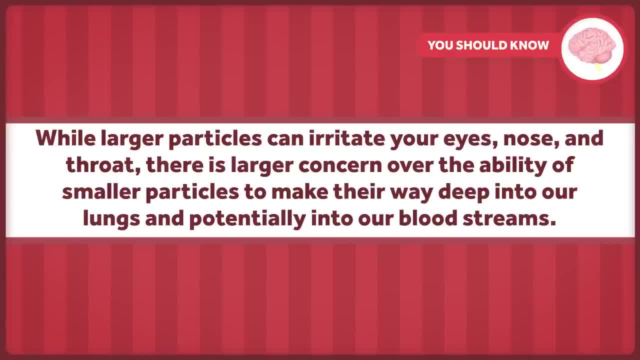 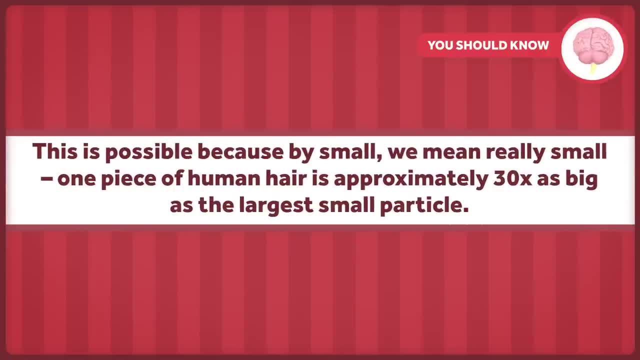 over the ability of smaller particles to make their way deep into our lungs and potentially into our bloodstreams. This is possible because by small we mean really small, and the thickness of one piece of human hair is approximately 30 times as large as the biggest. small particle. Long-term exposure to these small particles is linked to serious diseases, including lung cancer, stroke, chronic obstructive pulmonary disease and more. Emissions from wildfires, which are increasing in our warming planet, increase levels of particulate matter in the air, But according to some sources, climate change. 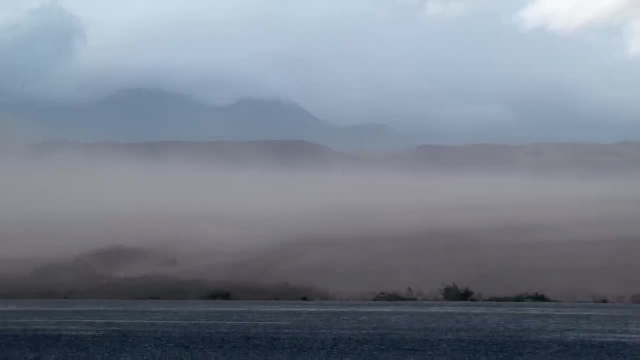 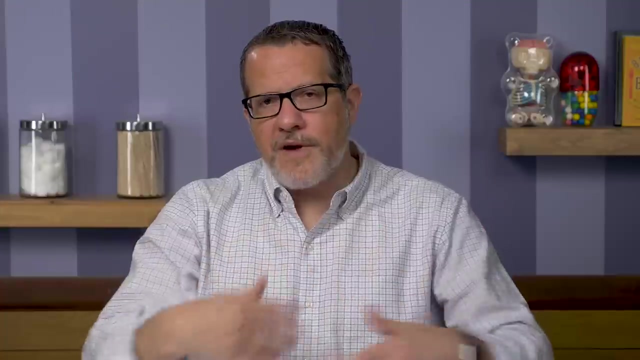 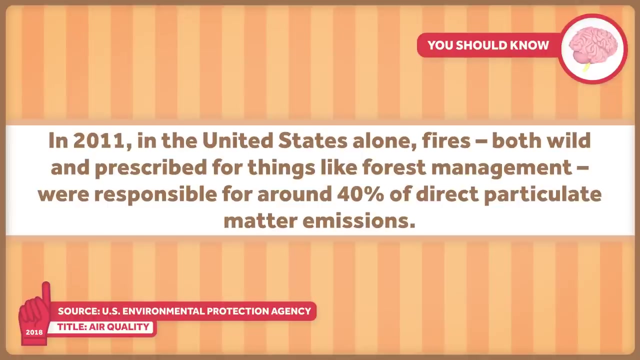 will lead to small increases in the concentration of particulate matter, even outside of wildfire emissions, and even these small increases can have big impacts on human health. But bringing wildfires back into the equation in 2011,, in the United States alone, fires, both wild and prescribed for things like forest management. 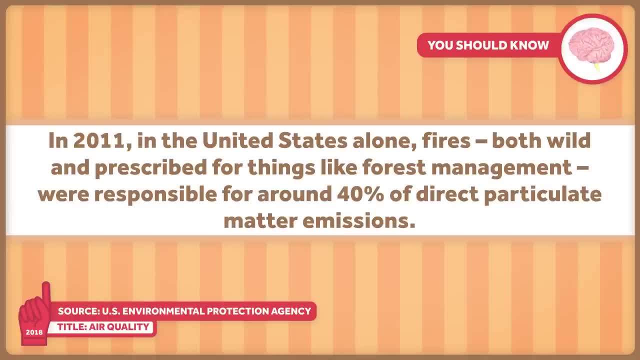 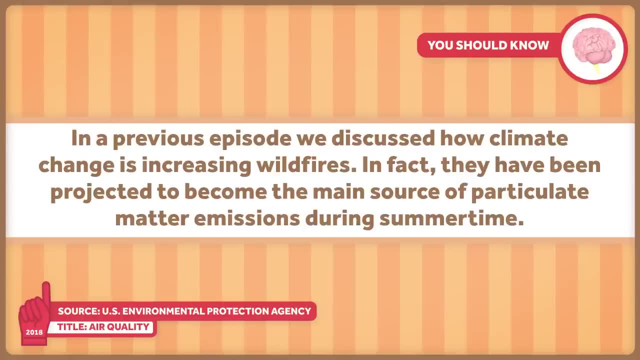 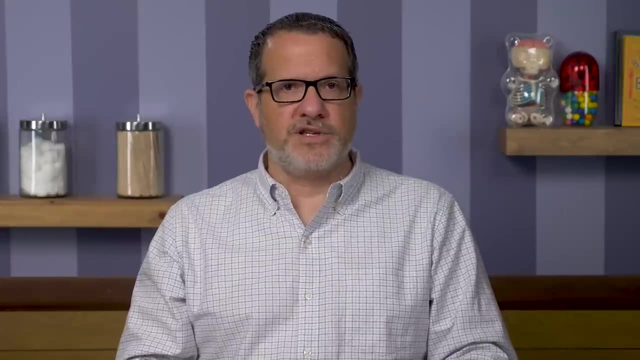 were responsible for around 40% of direct particulate matter emissions. In a previous episode, we discussed how climate change is increasing wildfires. In fact, they have been projected to become the main source of particulate matter emissions during summertime. Lastly, allergies stand to worsen with climate change, thanks to factors such as longer pollen. 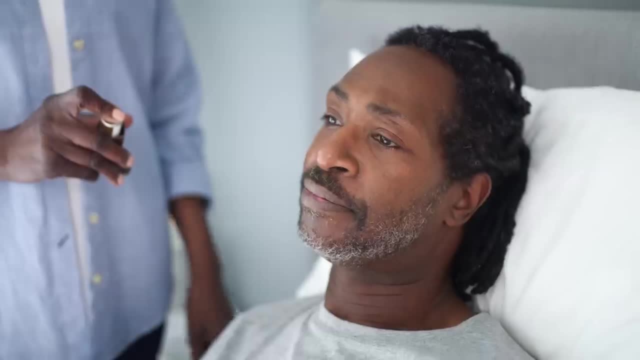 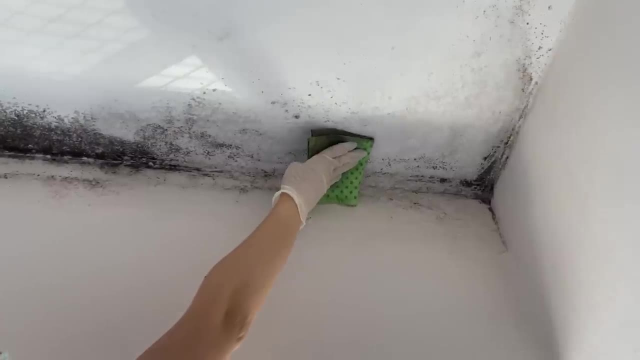 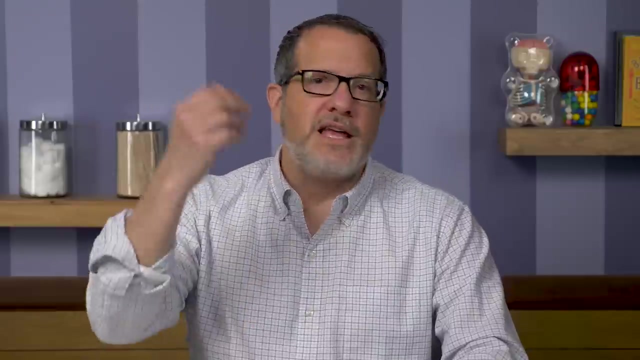 seasons and increased pollen production by plants. In addition, exposure to air pollution in combination with allergens can make allergic reactions much worse. Indoor air quality may also suffer thanks to increased heat and rainfall that contribute to problems such as mold growth. Alright, that's the end of our latest installment of the Hopeless Facts of Climate Change.